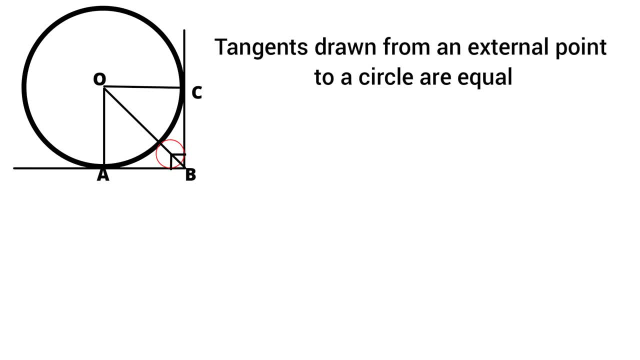 are always equal to each other Here. BC and AB are the tangents drawn from an external point B to that bigger circle. They also act as tangent to that smaller circle. So AB is equal to BC. Then OA and OC are the radii of that bigger circle. 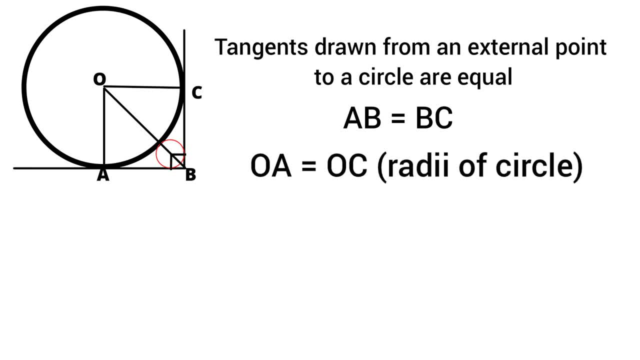 So they are also equal to each other. And we also know that tangents always makes right angle with the radius at point B, Radius at point of contact. So angle A is equal to 90 degree, Angle C is equal to 90 degree. 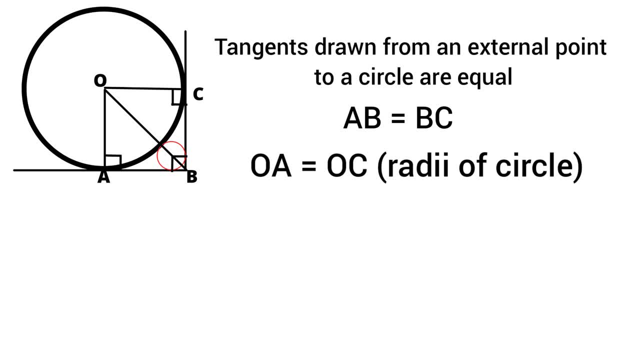 And also it is already given that angle B is 90 degree. Therefore OABC is a square of side length 2 cm. Now we can easily find out the hypotenuse OB value By Pythagoras theorem. we can write in right angle triangle: OAB. 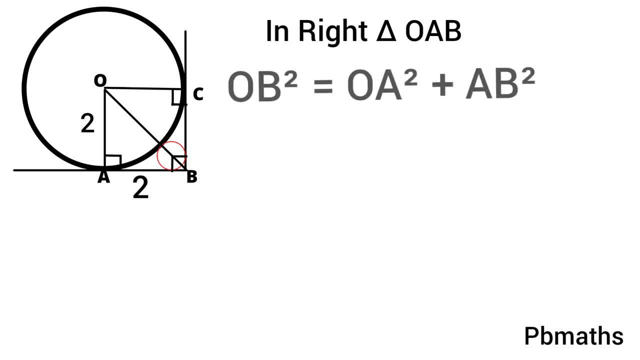 OB square is equal to OA square plus AB square, Which is equal to 2 square plus 2 square, Which is equal to 8.. Then the value of OB is square root of 8.. That could be written as square root of 4 into 2.. 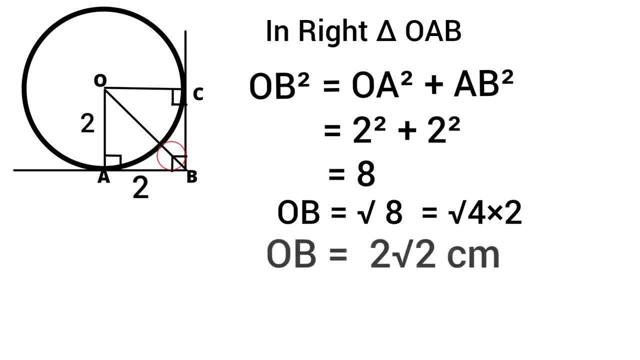 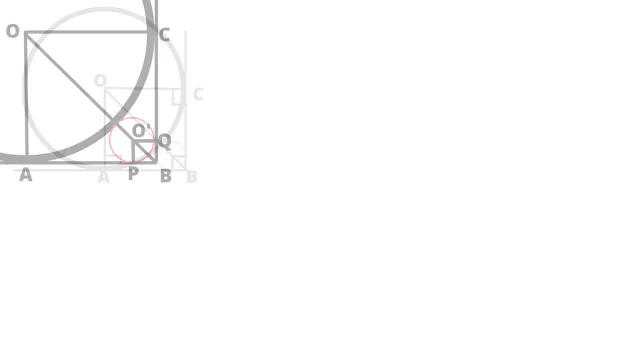 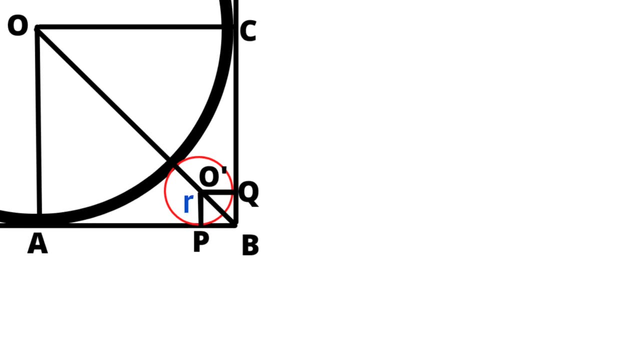 Therefore, length of OB is equal to 2 root, 2 cm. Let's zoom into that smaller circle. Let's consider its center as O' and radius B R. Let's draw two radii, O'P and O'B And O'Q, to that smaller circle. 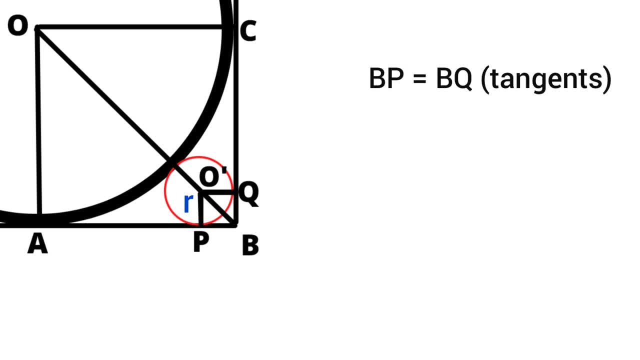 Here BQ and BP are the tangents drawn from that external point B to that smaller circle Which makes right angles at P and Q. Therefore O'PBQ is also a square. Then by Pythagoras theorem we can write: 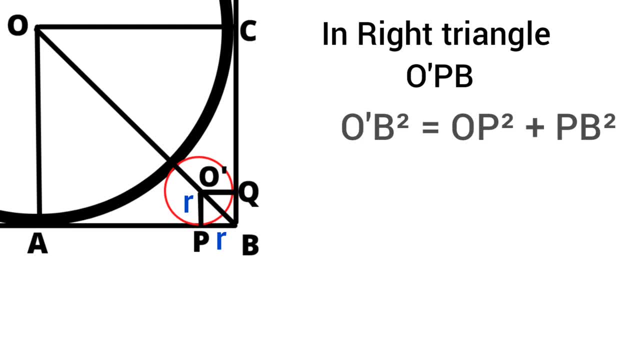 O'B square is equal to OP square. OP square plus PB square. Length of OP is R and the length of PB is also R, So R square plus R square is equal to 2 times of R square. O'B is equal to square root of 2 times of R square. 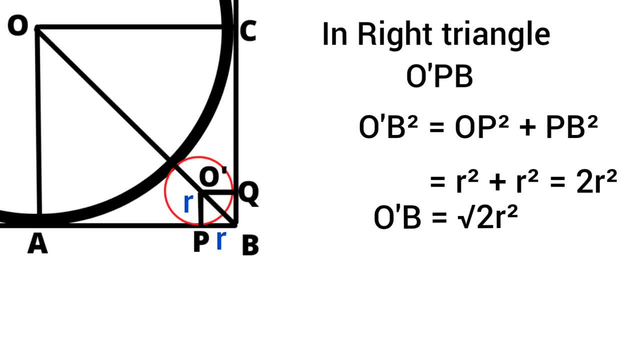 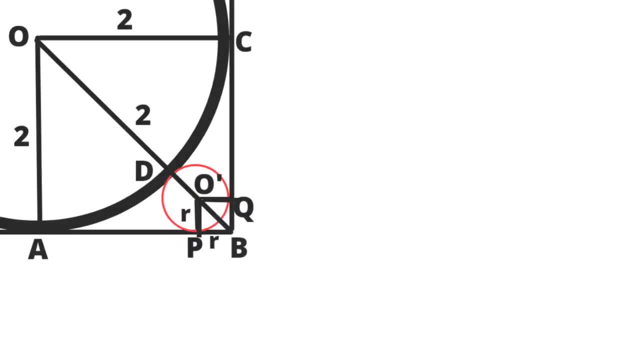 So the length of O'B is equal to R times root 2 cm. So the length of O'B is equal to R times root 2 cm. We already know the length of O'B, So O'B is equal to: We can write. 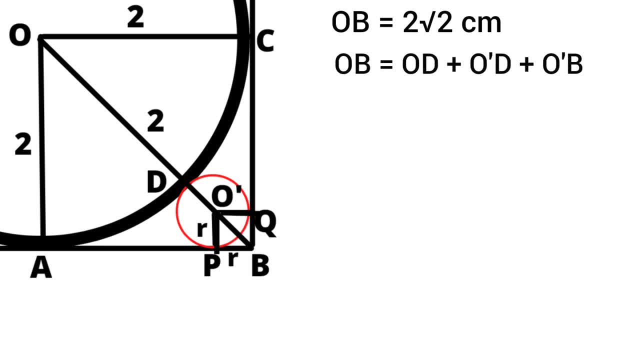 O'D plus O'D plus O'B. Length of O'B is 2 root 2 cm. So 2 root 2 cm is equal to: O'D is the radius of the bigger circle, Which is of 2 cm, Plus O'D is the radius of the smaller circle. 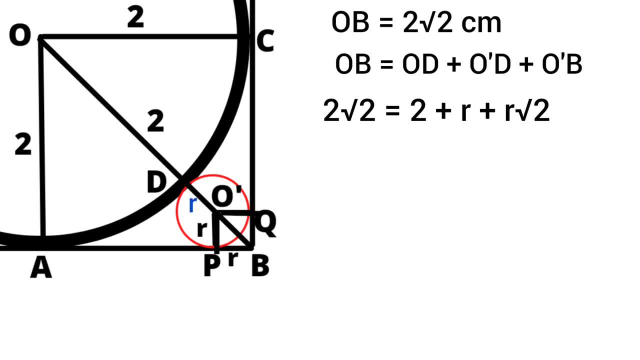 Which is equal to R Plus length of O'B, is R root 2.. Then R plus R root 2 is equal to 2 root 2 minus 2.. Then R times 1 plus root 2 is equal to 2 root 2 minus 2.. 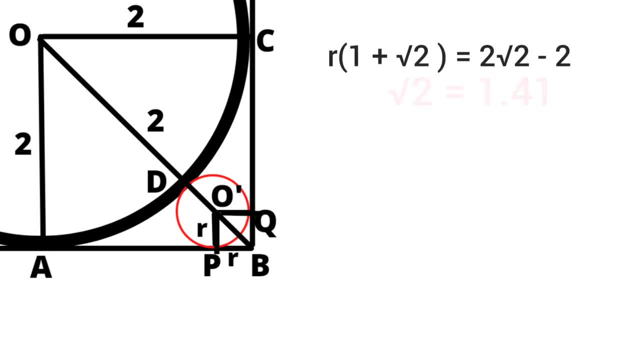 Let's consider the value of root 2 as 1.41.. Then R is equal to 2 into 1.41 minus 2 divided by 1 plus 1.41.. Which is equal to 2.82 minus 2 divided by 2.41.. 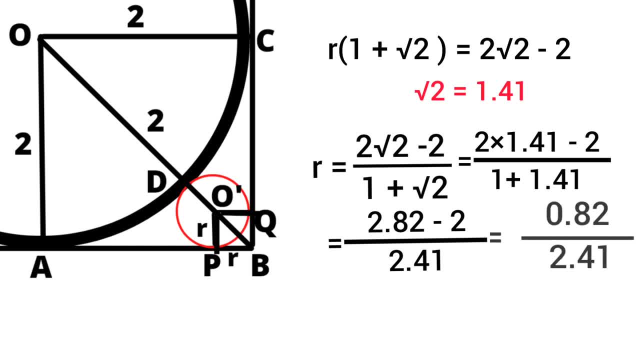 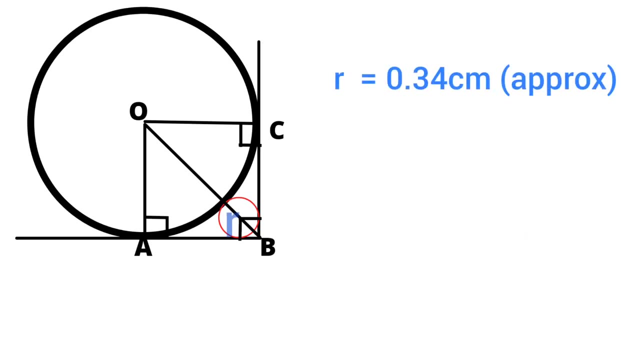 Which is equal to 0.82 divided by 2.41.. So the radius of the smaller circle is approximate to 0.34 cm. That is the solution. I hope you got this solution. Thank you for watching the video.